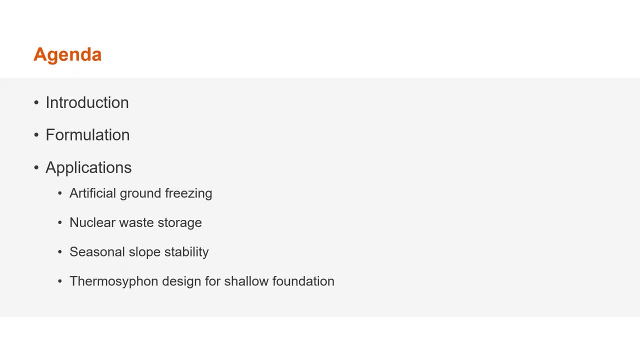 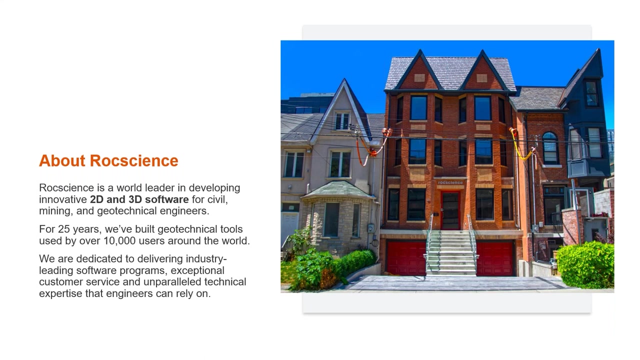 applications such as artificial ground freezing, nuclear waste storage, seasonal slope stability and thermal siphon design for silo foundations will be presented. As you know, RobScience is a world leader in developing innovative 2D and 3D software for geotechnical engineering in mining civil applications. For 25 years we have built 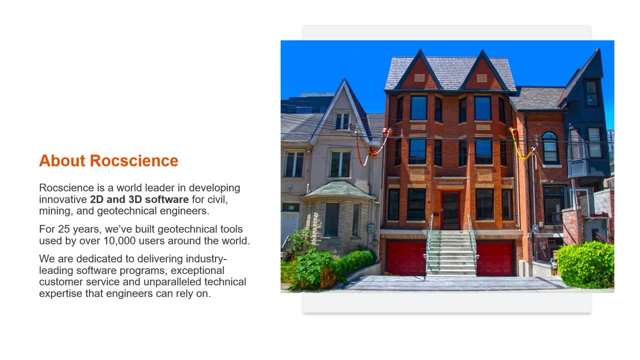 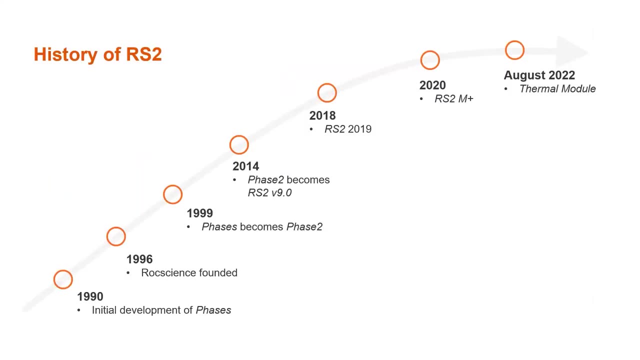 tools used by over 10,000 users around the world. We are dedicated to delivering industry-leading software programs, exceptional customer service and unparalleled technical expertise that engineers can rely on. We started development of IHU programs, which at the time was called FACE, in the 90s. 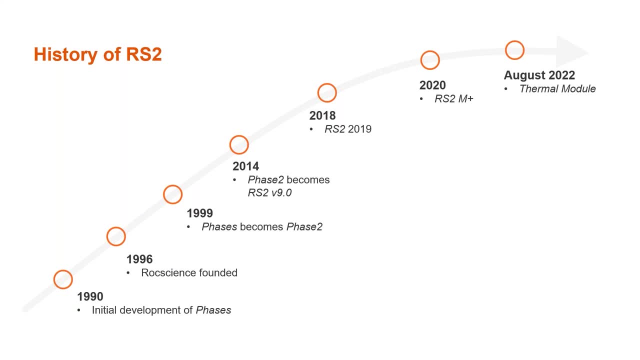 at a research group at the University of Toronto, And then in 1996, DropScience was found to provide various solutions for mining and civil engineering applications for the industry. Then in 1999, the name would change to FACE II. It would change because we started. 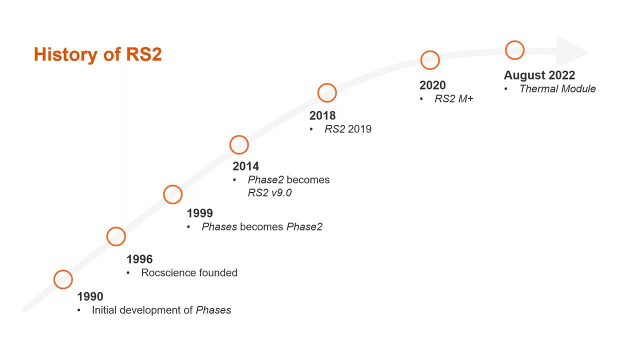 to develop a 3D version of programs, which you all know is IHU III, But at the time it was called FACE III. In 2014, the name would change to IHU in 2014.. And up to this version, we included: 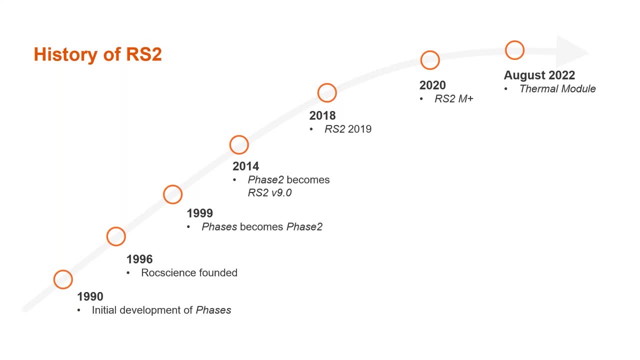 seed pitch analysis year constellations, dynamic community and many advanced constant models for soil and drought. Mplus were introduced in 2020 to provide more satisfactory customer support and new features to be included more often. We had non-sense of certain basic soil models. 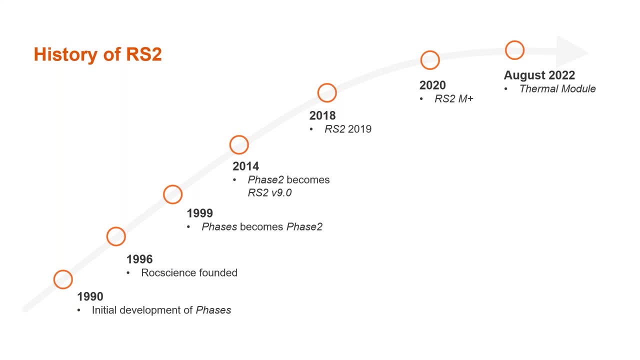 for unsaturated soil, vacuum constellations, relief wells, improved performance of dynamic analysis, including liquid fraction analysis, And in last month- August 2022,, we released thermal model which will enable IHU to run thermal hydromechanical coupling. 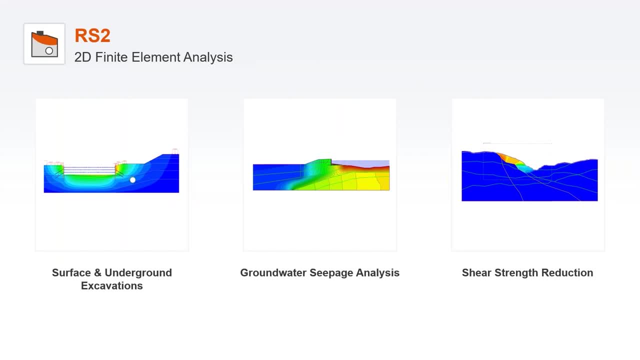 analysis. Generally speaking, IHU allow for analysis most of the geotechnical engineering design in soil and drought. Whether your project is civil or mining, based above ground or below, IHU enables you to effectively analyze straight deformations, stability support designs and stretch excavation with ease. 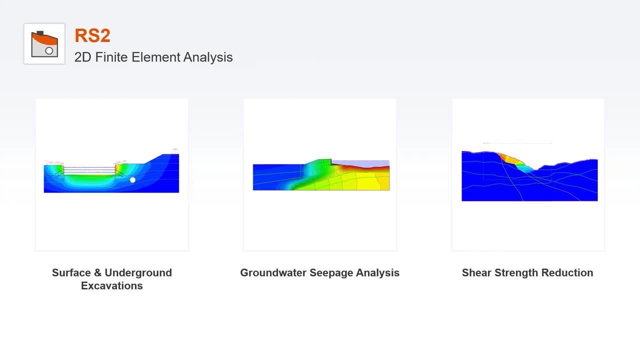 You can also factor in groundwater flow, which IHU integrated- seed pitch analysis, tools of steady state and changing conditions for dams, embankments, slopes, tunnel and excavation. And of course, you can also integrate with IHU and IHU also gain the ability. 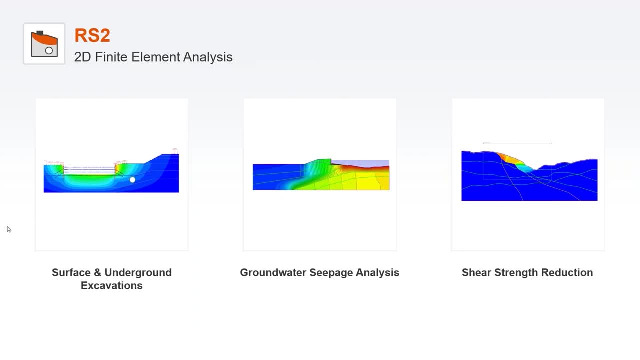 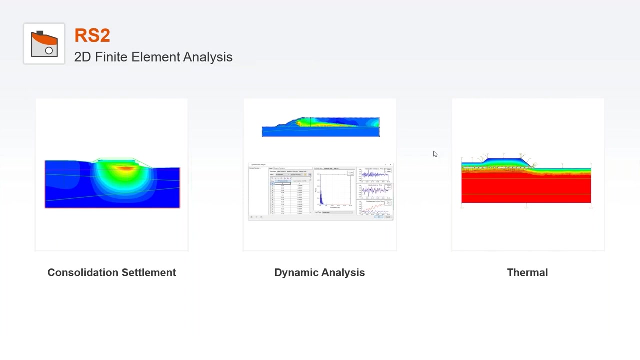 to automate the slope stability analysis with shear strength reductions which perform a finite element analysis to identify the critical strain reduction factor. It interprets seamlessly with LIHU programs which were proven the most slope stability popular program in the market. IHU also support consolidation of soil. 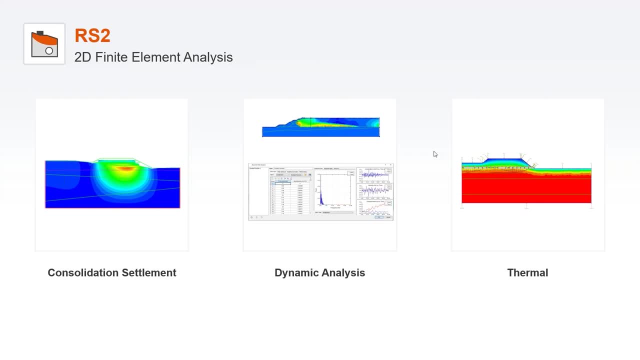 consolidation settlements, analysis for embankments, excavation and foundation designs. We also provide a lot of tools to use for dynamic analysis, such as natural frequency analysis, motion data processing and liquid fractions, And recently, with the additional thermal model, it enables IHU to analyze and evaluate the effects. 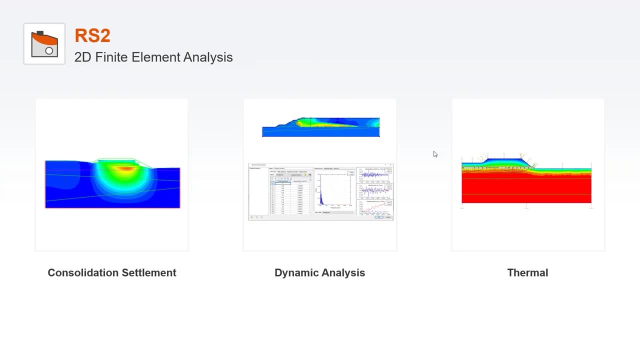 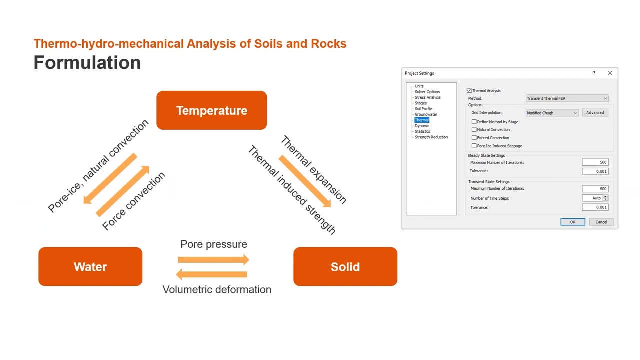 of temperature changes and to calculate the impact on the soil structure. By introducing thermal model now we can do fully couple of thermal, hydro and mechanical in IHU Temperatures. we have the effects on solids by thermal expansions and thermal induced strain defects. 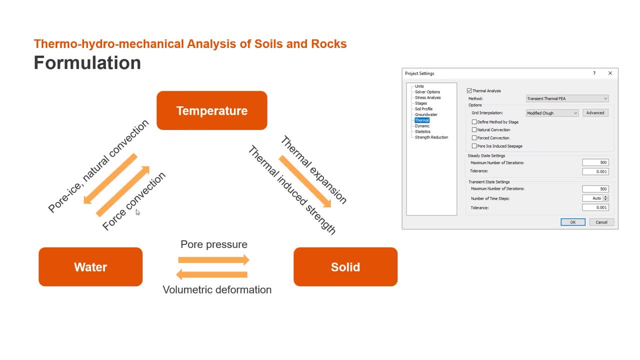 And rather we have effect on the temperatures by fault conversions, whereas the temperatures will affect the waters by the polarized behavior, natural confections or thermal-induced hydraulic properties And, of course, with the solid and water couples using the build couple approach. 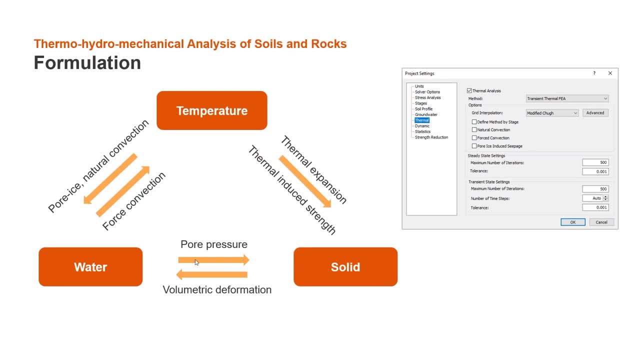 the interaction between water and solid will also be accounted for. Just a note here that we don't actually account for the effect of solid on the temperatures directly. We can, however, account for that effect indirectly to the effect of solid on the water and from the water to the temperature. 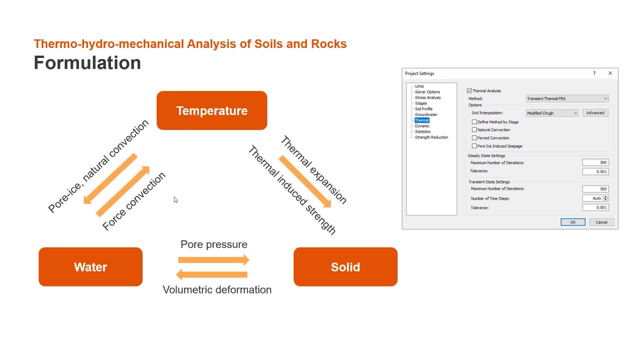 as you can see from the chart here, Thermal model can be activated in the project setting and you can turn on and off all of the desired behavior, such as natural confections, bulk confections or pool-eye-induced seepage, as you can see here. 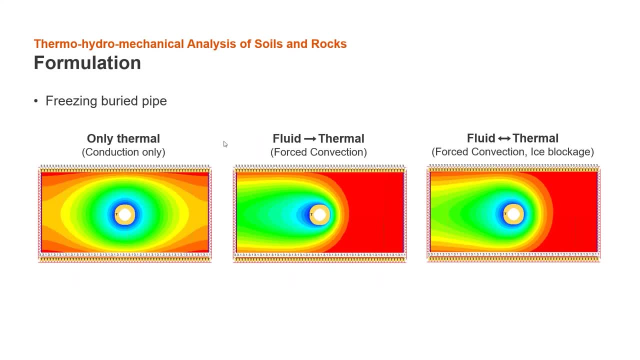 And here is a very simple example to show the interaction between the fluid and thermal phases. Three models were created to model the effects of frozen pipe on the surrounding environment and the water flow from the right to the left. for the two models that we have the fluid effect on. 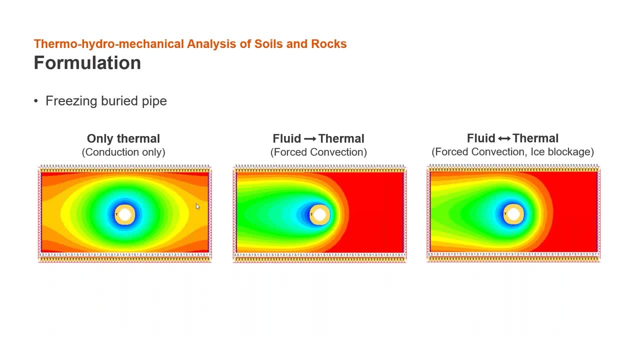 The first one only consider the thermal conduction only. The second one when we have the effect of the fluid on thermal one way And the first one when we actually activate both way, couple between the fluid and thermal. And, as you can see here on the first model, 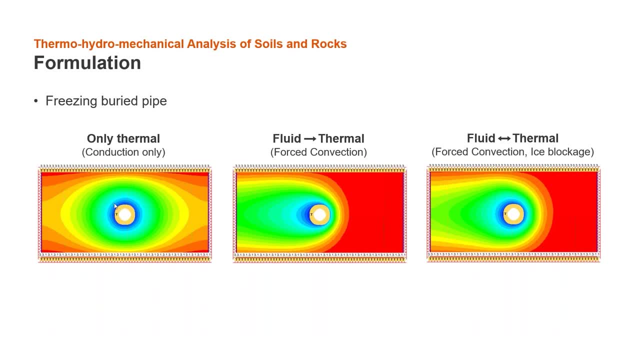 the temperatures around the freezing pipe is symmetric. However, because of the water flow here we can see that there is a massive. there's a minimal effect of the frozen pipe zone on the upstream of the models And when you account for the effect of the temperatures, 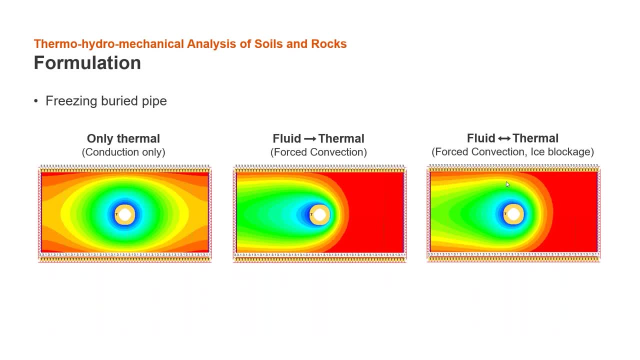 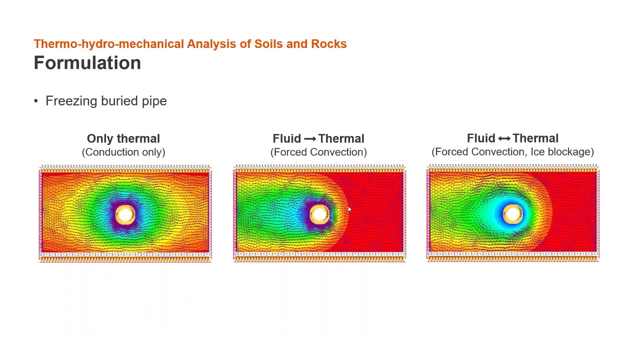 on the fluid we can see that there's a tension of the frozen zone vertically on the model, And here is the water flow in the model after the simulations. And on the third model, when we activate the both way couple, we can see that surrounding the frozen pipe. 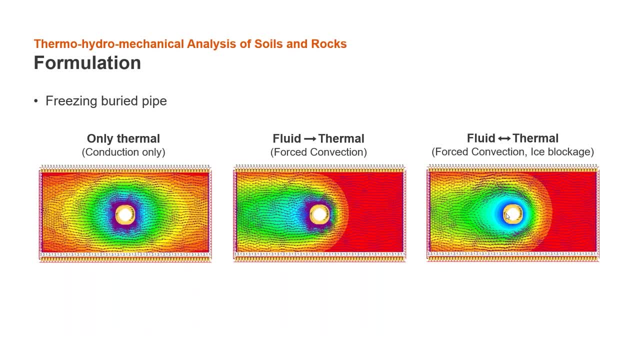 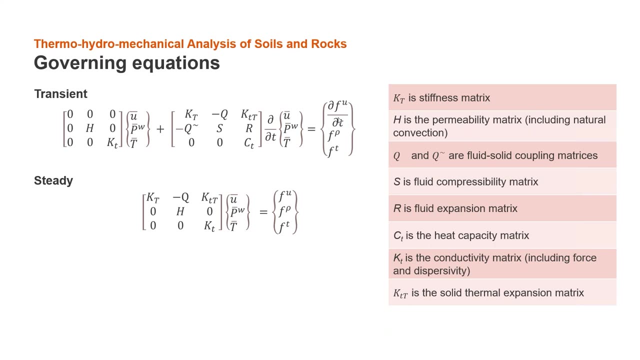 there's no water movement because basically all of the waters around the frozen pipe was frozen and no water can flow. And here is the math behind the scene, And I know that most of you will not be interested in this, So I just go very briefly about this. 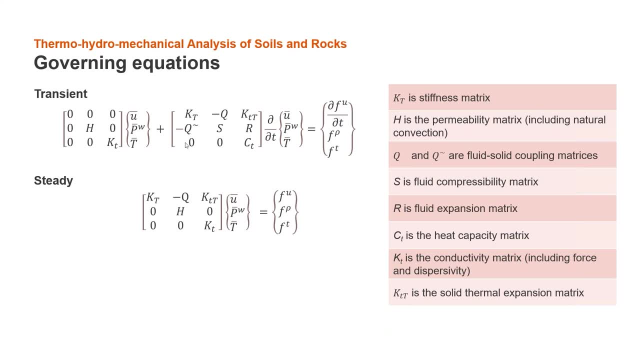 But here's the equation: that we put everything together To get the zone, to get the effect of temperatures, fluid and deformation all together. And the convection term- here accounted for the heat transfers by water flow- is included in the KT here, which is the conductivities matrix for the thermal term. 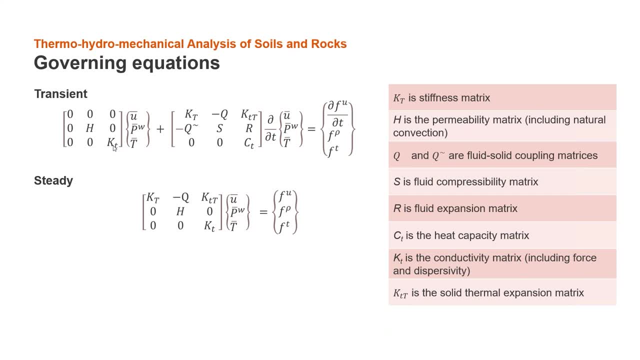 And, moreover, with the water content changing, the thermal property can also be changed depending on the flow, So depending on the thermal model that we use. also, the permeability matrix H and the compressivity matrix also include the function of temperature, permeability and water contents. 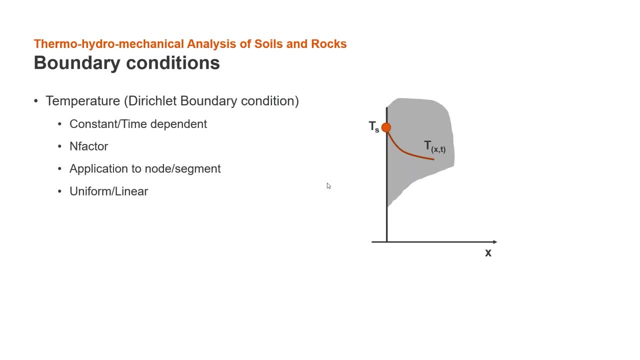 We also provide many battery condition type that can be used for most of the application-informed thermals. Users can assign temperatures or the display battery conditions constant of temperatures. it can apply to node or segment or it can be uniform along the surface shear. 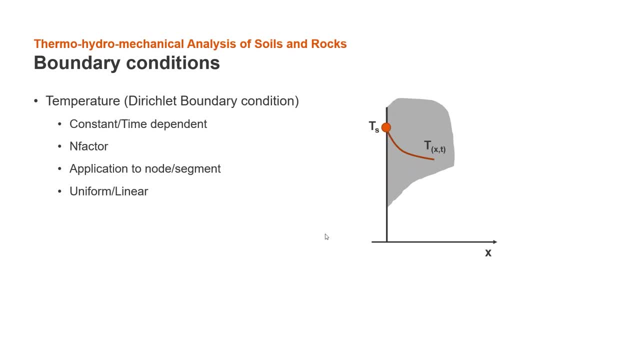 or it can be very linearly along the surface. You can also assign n factor to offset the temperature that actually applied on the surface. A second type that we provide is the heat plus or normal type that can be assigned to node or segment as well. 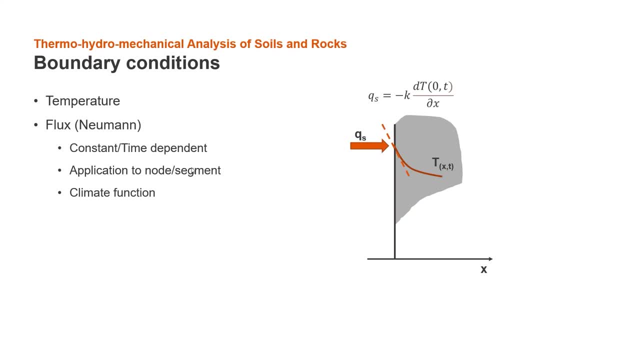 It can also be a constant or time-dependent. We also provide climate functions where it can be called a surface energy balance, where the effect of solar radiation, vegetation, snow cover, wind speed, air temperature can be accounted for all together. Note that when you don't apply the first body condition, 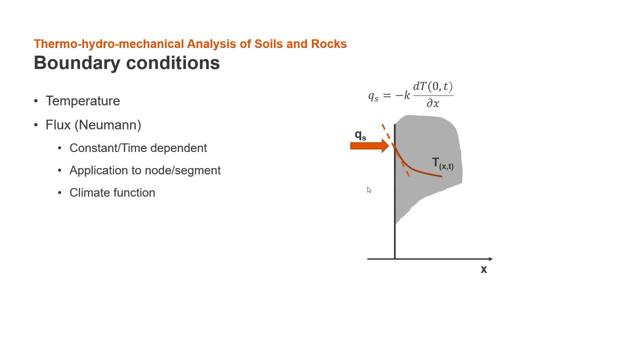 on the surface and there's no temperature battery condition. it is a special case called the perfectly insulated surface, which means that there will be no heat in and out from the surface. We also include the convection-barrier condition, where we can account for the heat transfer. 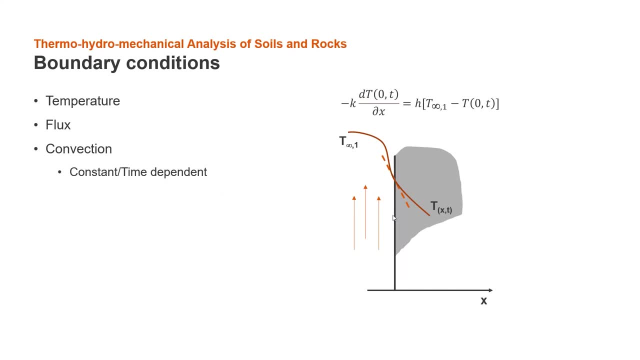 between the two medium. For example, you want to account for the heat transfer between the air and the solid, or you want to account for the heat transfer between the fluid and the liquid And the solid space as well. We also provide the insulations of a thermal contact. 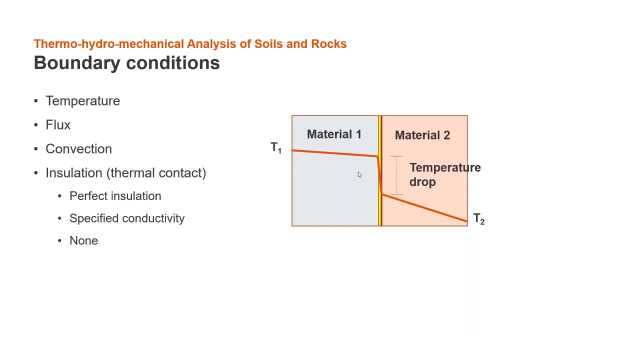 As you can see here in the figure, there's thermal contact between the two materials here And you can either specify it as a perfect insulation, or you can specify the conductivity for the thermal contact, or you can select none, which means that the temperature 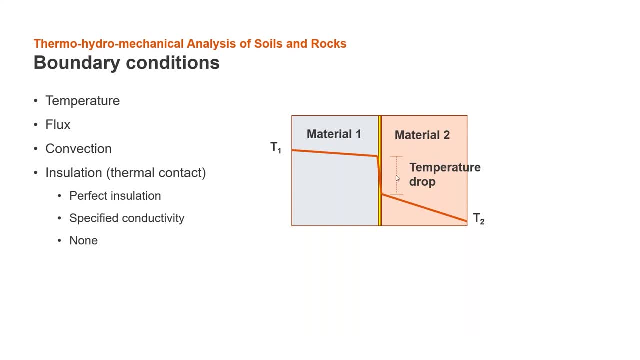 as you see here, for the temperature drop it could be equal to zero when selecting none here, And for the perfect insulation, the temperature between the two materials are not related at all, Or you can control the temperature drop here by specify conductivity or thermal conductance. 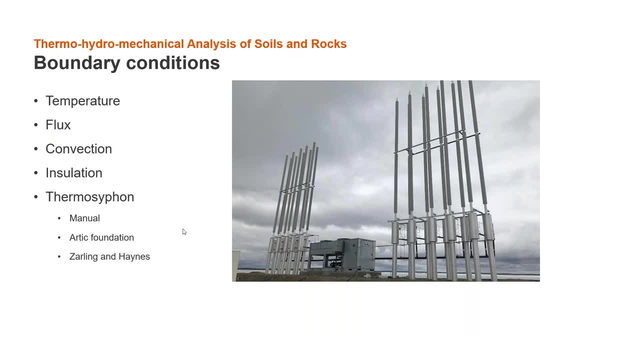 Another body condition we provide is thermal siphon, and thermal siphon means the thermal contact between the air and the liquid. Thermosyphos was widely used since 1960 in the Arctic climate, where soil freezing is accomplished passively. 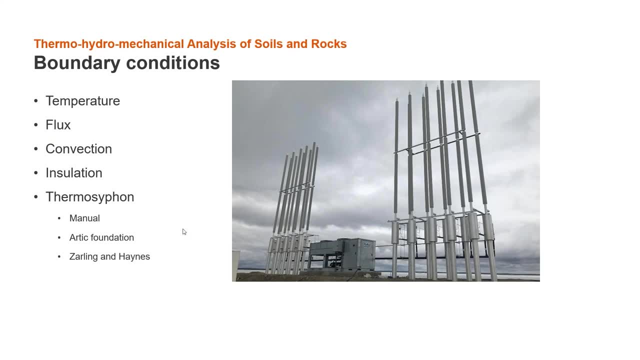 For example, you don't need to use any power to run the system And they can be assigned automatically in IHU. User can have three options to do that. You can either assign manually or use already established methods such as Arctic foundation or zealot-enhanced method. 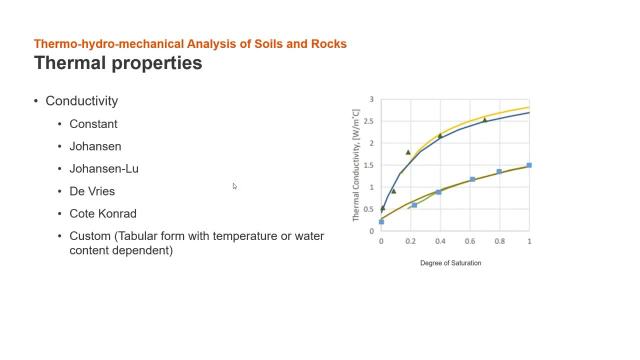 We also provide many methods to model the behavior of the soil in thermal analysis And, for example, for the conductivities. you can have constant, you can have Johansson's or Johansson and Lue, You can have every pot and crud And of course you can have the. 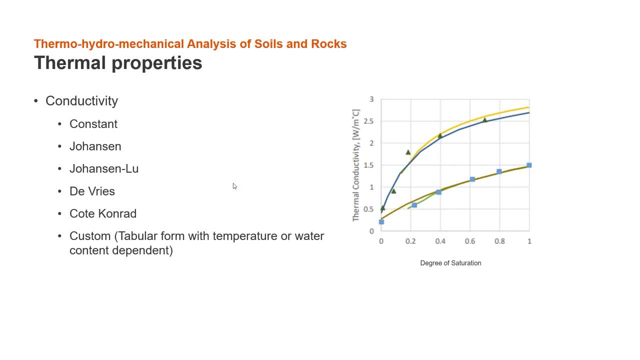 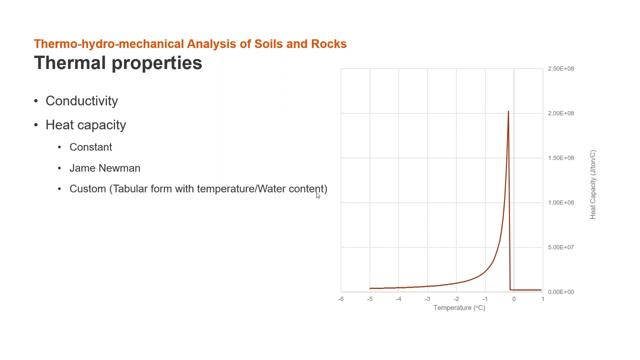 custom type, which means that you can input the conductivity manually, dependent on the temperatures or water content. And here is the typical thermal conductivity, changing with the variation of degree of saturation, as you can see here in the graph. And another very important properties of thermal analysis is the heat capacities. 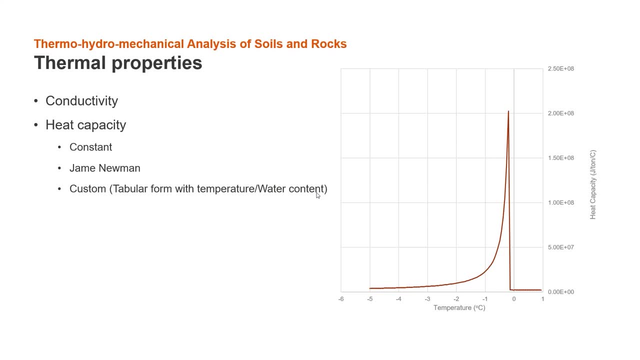 We have three ways to model heat capacity in IHU. You can have constant heat capacity, you can have Jem Newman's method and, of course, you can do it as a customer Using the Jem Newman method. our effects of ice water and solid Contribution to the 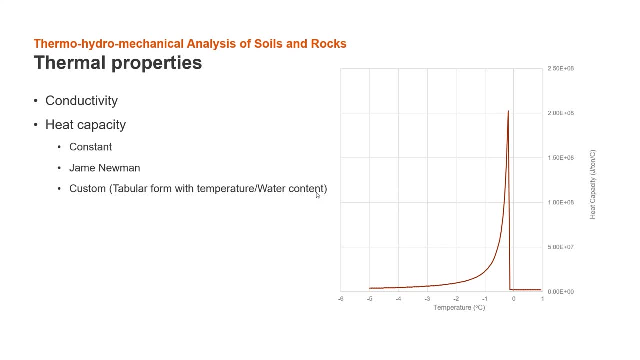 the heat capacity will be automatically accounted for. You can also specify to include the latent heat or not. So, as you can see here in the figure on the right-hand side, as the temperatures approaching the freezing point, which is close to zero here, 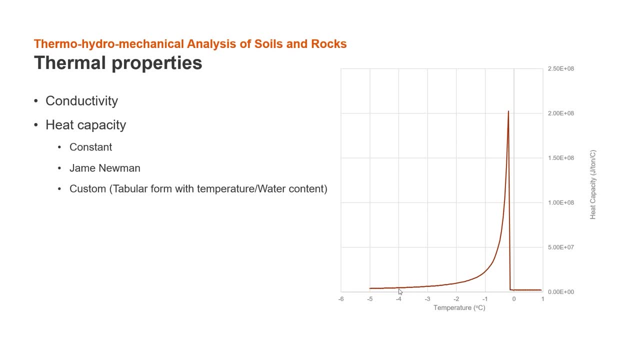 the heating capacity of the material increase exponentially And because in that model we accounted for the latent heat right And this is causing a lot of issue in conversion- when we accounted for the phase change in thermal analysis. Traditionally this behavior required a very long time step. 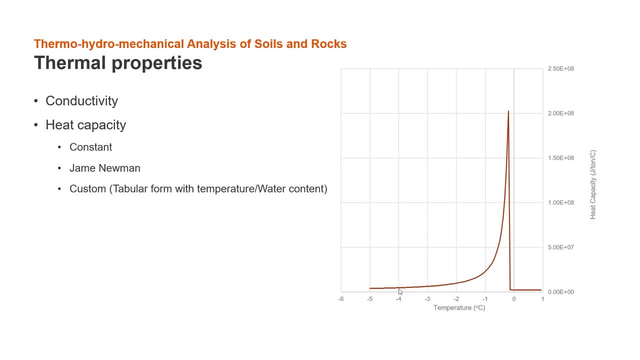 to capture the front face correctly. However, in IH2, we developed an on-topic comparison that says in scheme that it will always capture the energy correctly from the phase change behavior, And so you can use much larger time step without worrying much about the accuracy of the results. 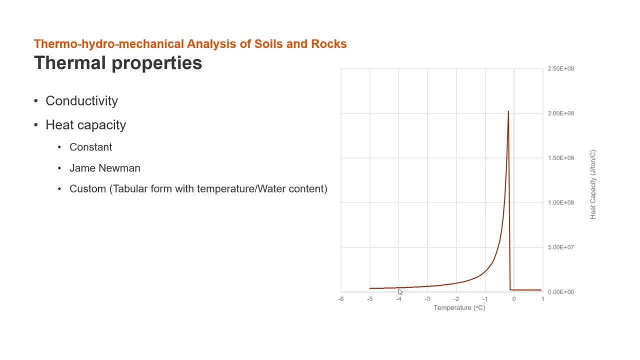 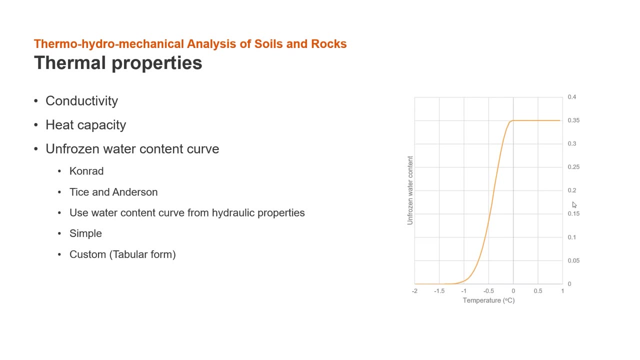 It also results in the excellent conversion rate as well, And one of the most important characteristics when modeling thermal in soil or rock is the unfrozen water content curve And it's extremely important to calculate the effective conductivity, effective heat capacity, And it's also very important to capture. 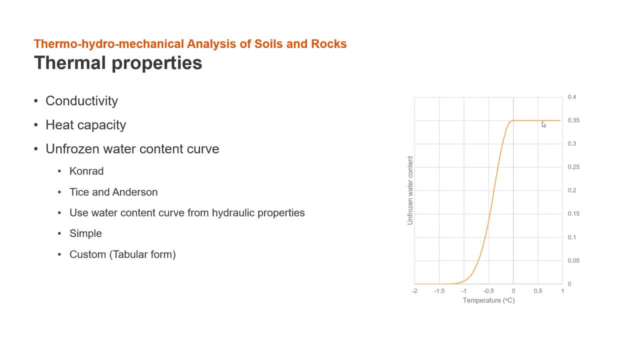 the phase change phenomenon in geomaterials. And here is the typical unfrozen water content curve for soils. And you can see here at the soil temperature is less than 1.5, minus 1.5.. The unfrozen water content is zero. 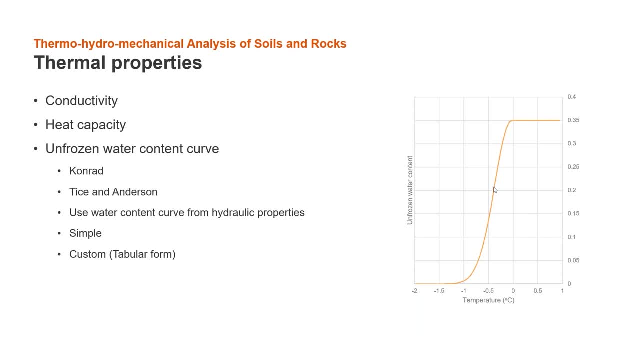 whereas it keeps increasing as the temperature increase And when the temperatures are above the frozen point and the unfrozen water content will be equal to the water content of the saturated value, And we provide several methods to do that. You can use methods from CONRAD or TIE and EDANS. 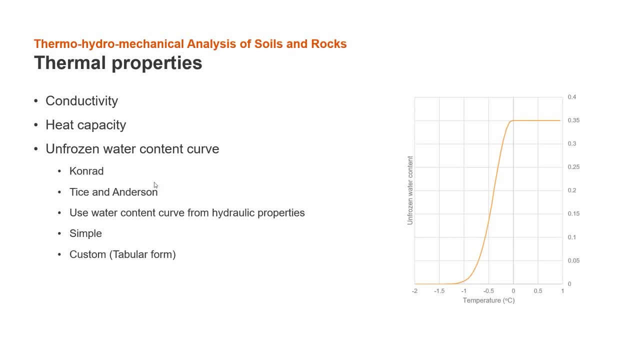 you can even use the water content curve from the hydraulic properties such as van Nusselt, or you can use a curve from FETLIN and SYNG- you name it- And so the question here is that many of you may not have enough data to have one of these fancy model. 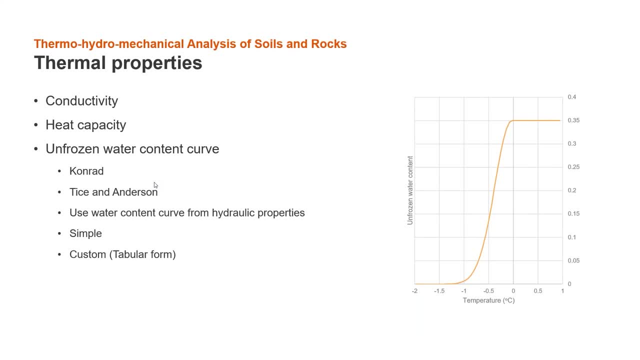 available and you only need to and you're only interested in the various, you know- simple simulation to see how it behave. So we also provide a simple model here with the, which is only required one single parameter, which is the frozen temperatures. 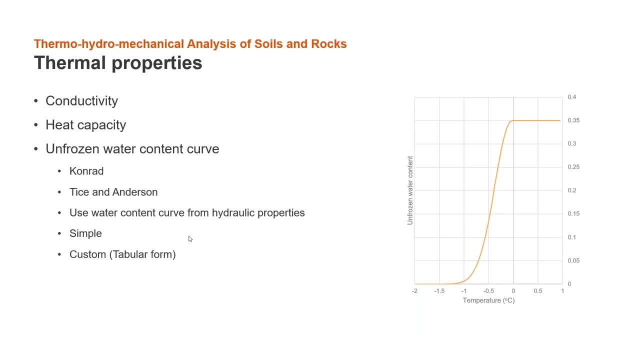 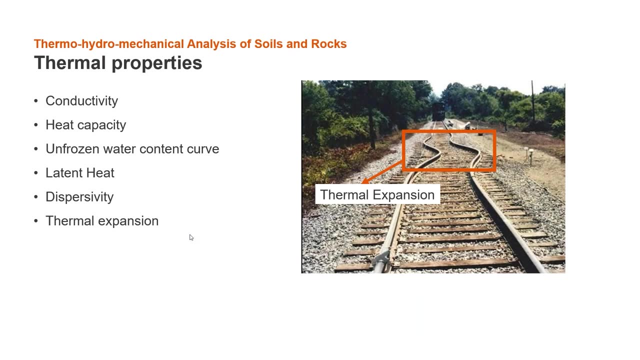 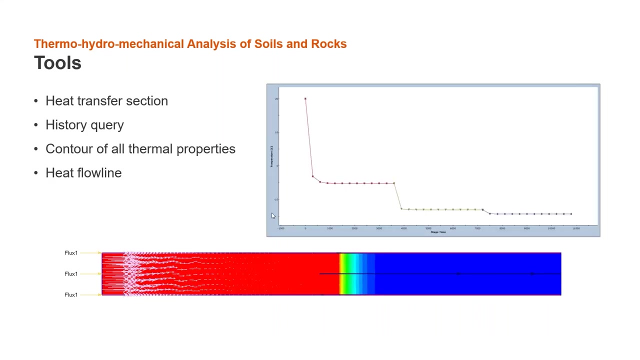 And you can also input it manually using the tabular form as well. And we also have the capability to account for the thermal, the specificity and thermal expansion of the core, So you can see how much heat was transferred to the sections using the heat transfer sections. 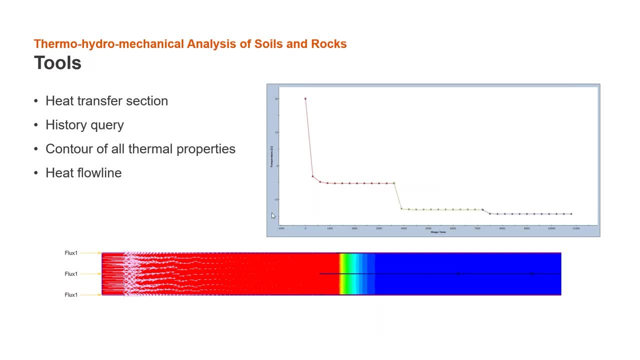 After the cleaning is completed, you can easily see how much heat was transferred to the sections using the heat transfer sections And all of the thermal properties such as conductivity, heat capacity, unfrozen water content and thermal results such as temperatures, heat flux, heat gradient, heat flow length can also be visualized by HETROL. 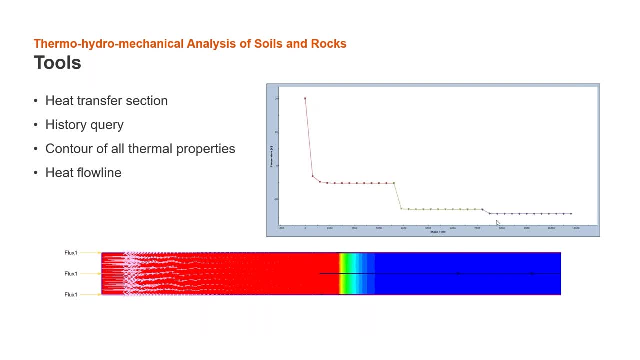 And that's something that you can do by controlling as well as the history query, as you can see here. For the history query, you can also visualize, during the calculation as well, to our engine GUI where you can see the temperatures, the placement. 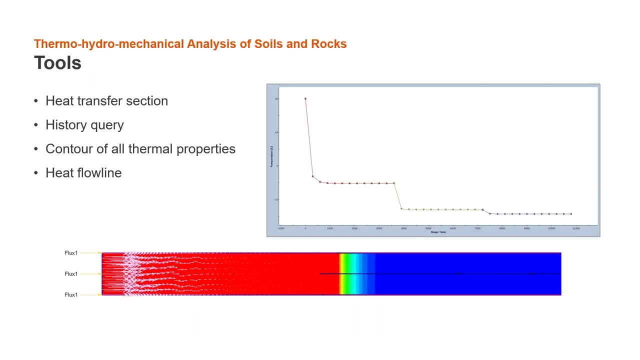 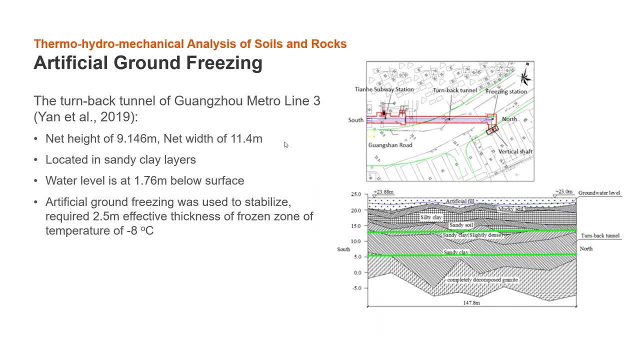 purpose of changing during the calculation. So the first application example, the artificial ground freezing or AGF Ground freezing perhaps, is one of the most popular ground support methods in mining and civil and environment project. even It is sometimes the most preferred methods because it's low impact to the environment. 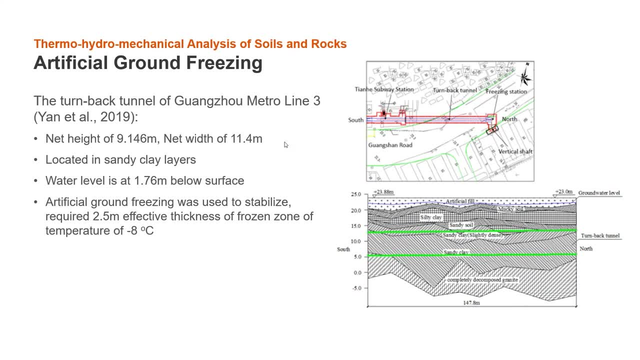 And in this typical example I actually will use to back analyze an artificial ground freezing design for a turn back tunnel of Wanzhou Metro Line 3, based on the paper obtained in 2019.. The tunnel has the height of nine meters and the width of 11 meters. 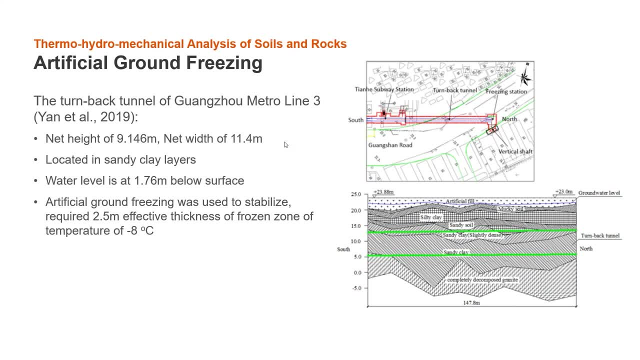 It's located in the sandy clay layers four meter below the ground surface that you can see here, And the ground water level is at 1.76 meters below the surface. The requirement of the design is that the effective thickness of the frozen zone had to be 2.5 meters. 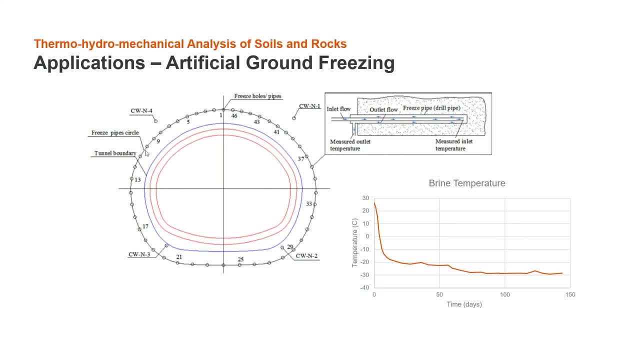 And in order to achieve that, they have been installed a series of the pipe outside of the tunnel battery, Here, the tunnel battery that you can see here and here is the series of the pipe here And the bright was pumped to the closed system from our freezing stations and the temperatures. 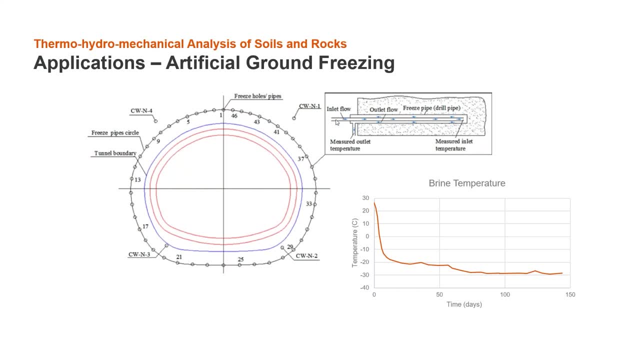 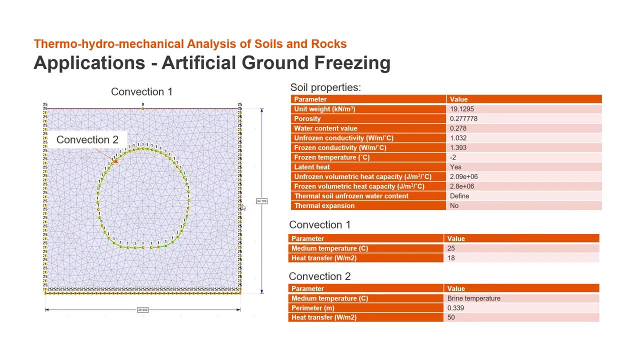 of the inlet and outlets will measure and the bright temperatures will control to achieve and maintain that frozen depth until the design support will install. And here is the bright temperatures from the paper And here's the model in IHU. So here we only pay attention to the thermal design. 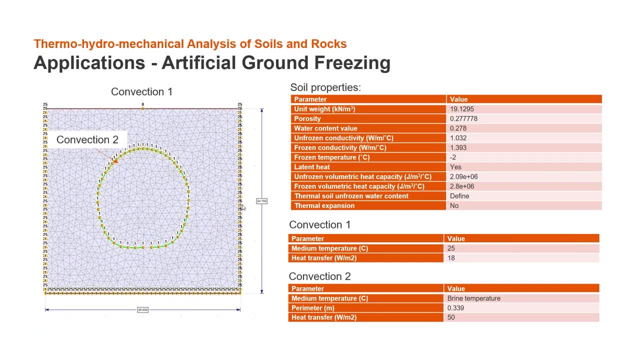 So we did not want to be over complicated the model And we just so we didn't account for the dry water level. But instead of doing the full seepage analysis here, we just need to set the water content value to 0.27H, which is equivalent to the prostate of the material. 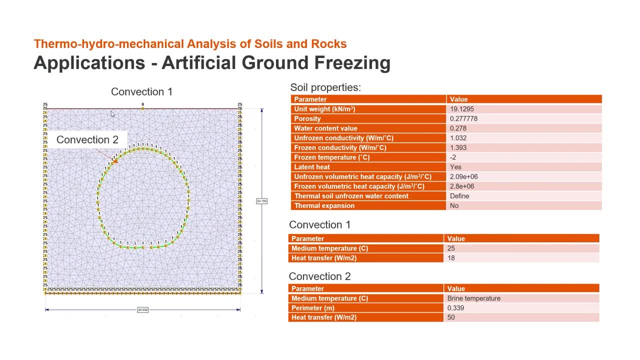 The convection barrier condition will assign at the water content value to 0.27H, which is equivalent to the porosity of the material. condition will assign on the top to represent the interaction between the air temperature and the soil, And the brine or the frozen pipe was modeled using the convection barrier. 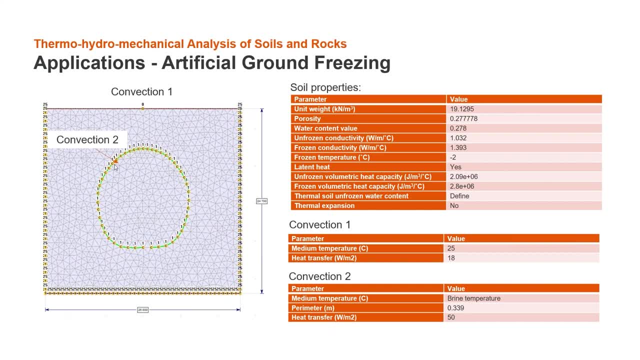 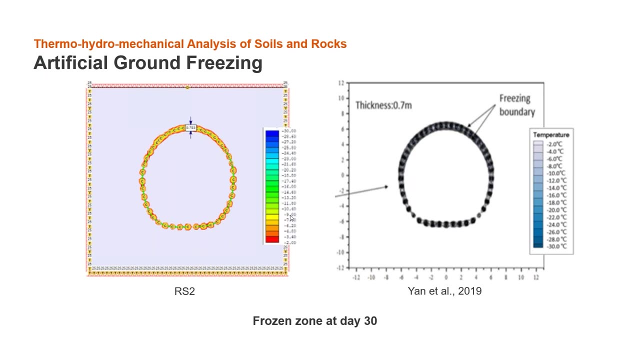 condition as well as in the convection number two here, And the medium temperatures were assigned with the brine temperature as shown in the previous slide. And here are the frozen zones calculated from the IHU and the results were compared with the results from the paper And you can see that the zones are very similar at the day. 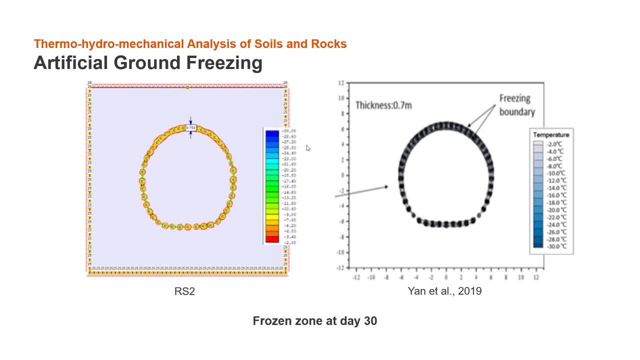 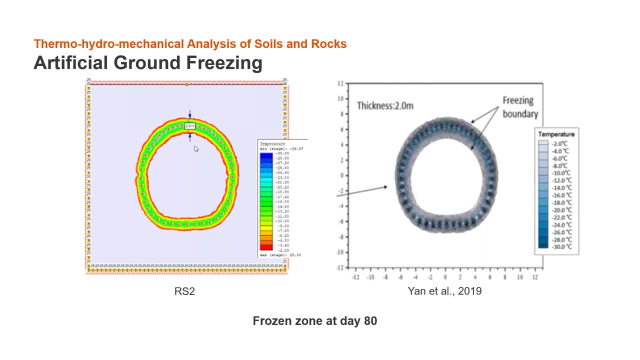 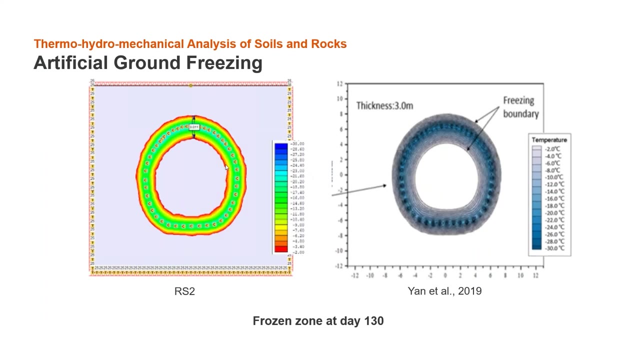 30 with the thickness of 0.7 meter. A very similar behavior was observed at the day 80 as well, where we have the thickness of 2 meter in the most IHU in the paper And the thickness of 3 meter were achieved at the day of 130.. And the same behavior was. 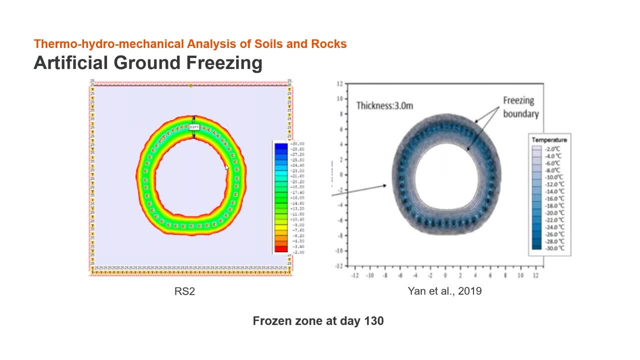 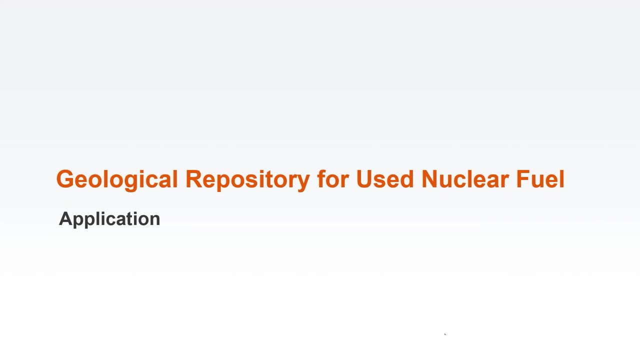 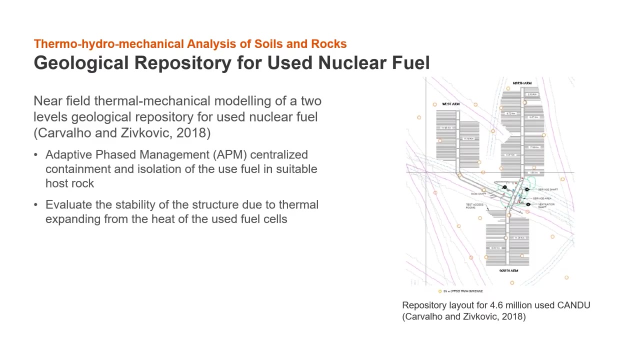 seen in IHU and the paper as well. Another example I'm presenting today is to evaluate the stability of geologías, repository of used nuclear fuel. In this example we back calculate the designed from Cavagno and Zikovic for nuclear waste management organizations for long-term. 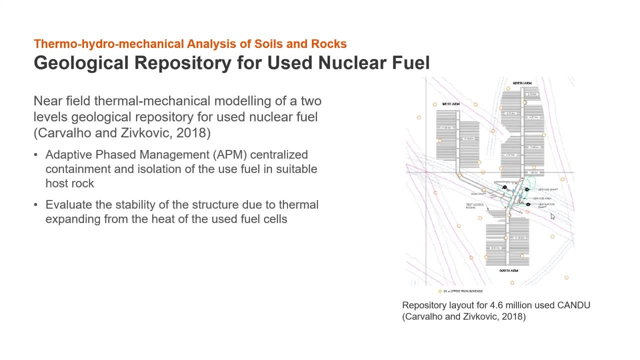 management of Canada's used nuclear fuel. The layout of the repositories was shown on the right side, as you can see here Also. the fuel cells are stored at two levels, approximately 2.3 million spindles per level, with a lower level start 20 years after the start of. 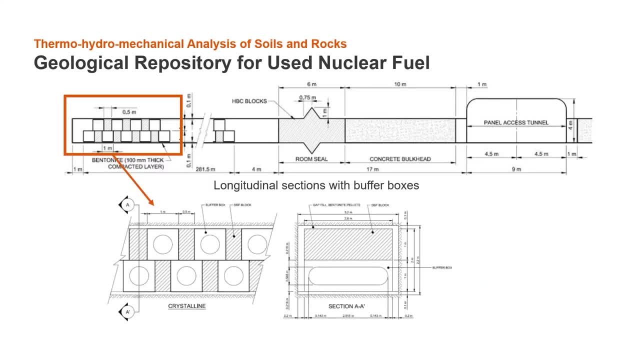 the first level Here is the longitudinal sections with buffer boxes, The center to center distance between the boxes at 1.5 meters and between the boxes at 0.5 meter of the buffer filled with bentonite pallets, And you can see that the top and the bottom rows are offset. 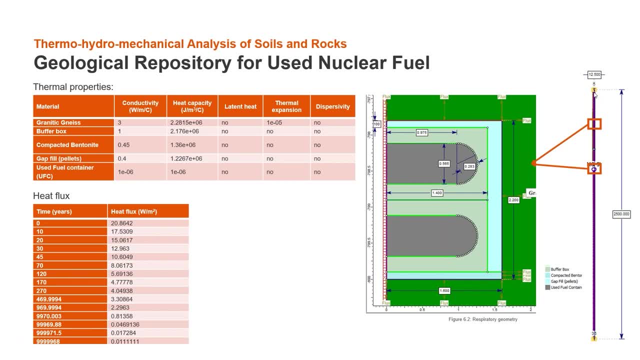 And here is the model in RSU We are doing the analysis for the case- that have 25 meters room spacing. The repository levels are located between 400 meters and 800 meters below the ground surface In this particular example, because the area of interest is far away from the ground level, so we don't have to include the effects. 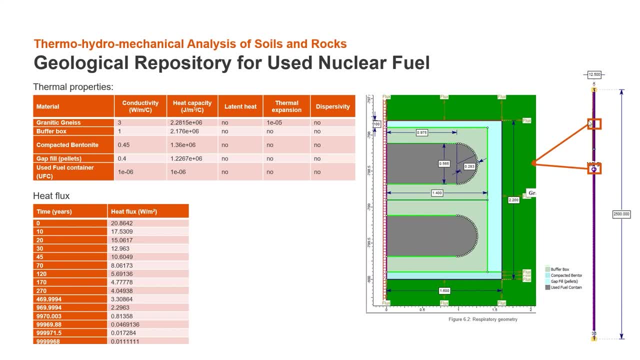 of climbers to set the computational load time. So the temperature of five will apply to the top And 35 degrees 00.65 tussen Märs lí, 381 H核 381 Kɸ was applied to the bottom. The initial temperatures will vary linearly along the model. 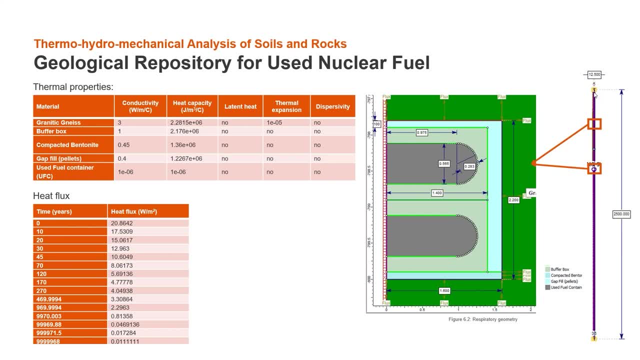 The heat flux for each box were calculated from Mark II use fuel cell generations as shown in this table And you can see that the heat flux degree by time and also, please note that the uses cells only placed after 30 years of the uses, So the value of the heat flux. 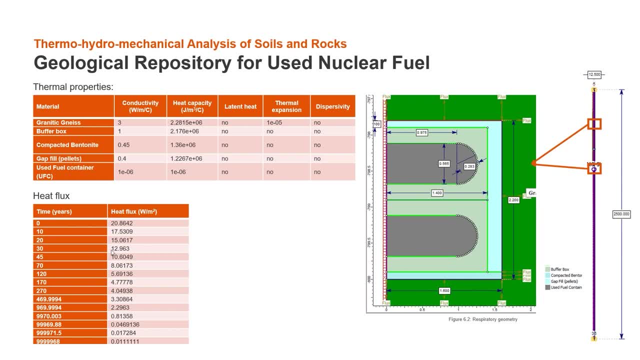 occur at the 30 years will be used for the installation stage And those value was all calculated from the Mark II use fuel heat generation source term. The drop was modeled using the hook brown materials and the thermal property was shown in this table And, as you can see here, the thermal expansions car efficient was 1E-5.. 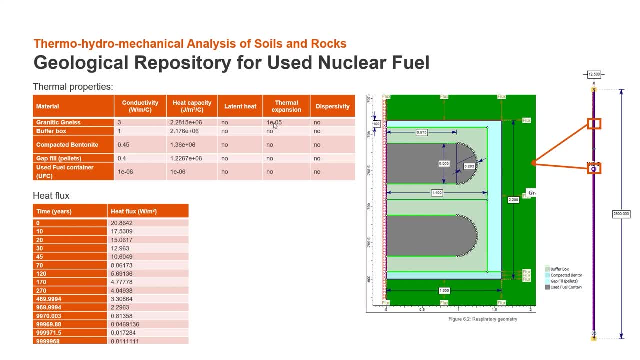 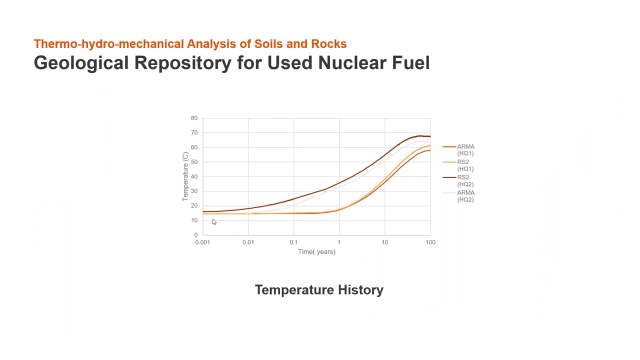 There are two conditions for the design to be acceptable. The first one is the temperatures must not exceed 100 degrees over the whole time, And the second one is the repositories had to be stable. And here is the temperatures development at the side edge and the center point. 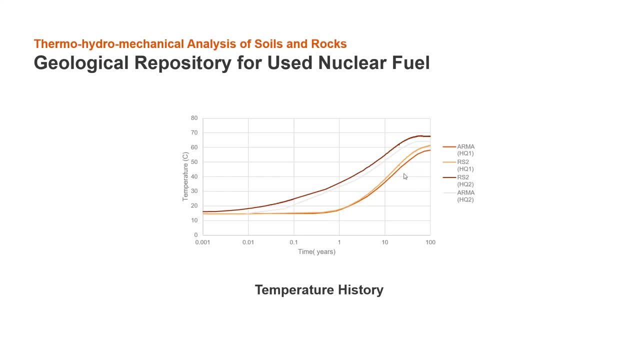 The side edge is the light red and orange here And the center points at the brown and the gray one lights here. As you can see, the result match pretty well with one from the paper. The temperatures at the center point rate immediately when the fuel cells were placed. 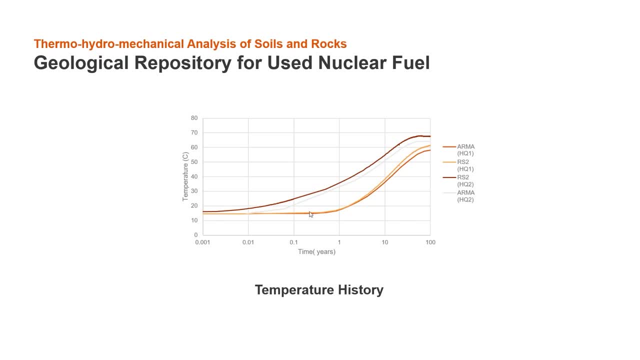 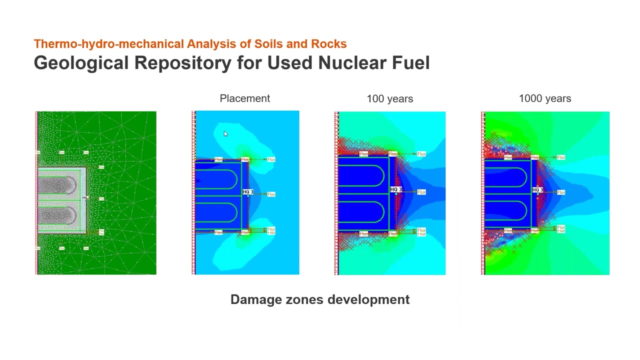 It took almost three months- for the edge points start raising the temperatures And after 100 years the temperature at the point are below 70 degrees, well below the requirement of 100 degrees. And here is the dynamic zone development induced by thermal expansions. 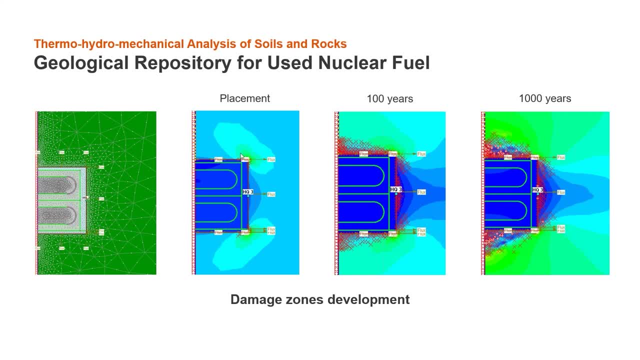 At the time of placement of the fuel cells. there are minimal of failures in the models, Only a little of shear failures happen at the corner of the repositories. However, as the temperature increases, the temperature increases Because the volumetric strength induced by the thermal temperature change. 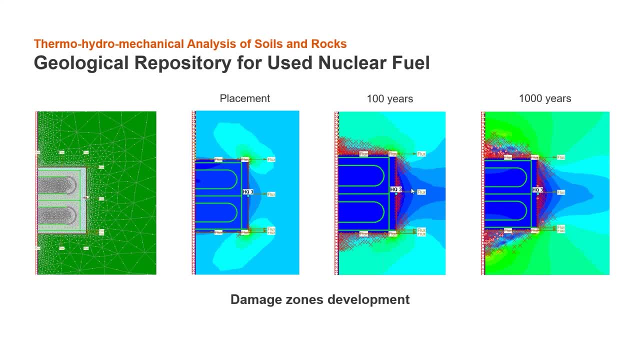 And we're going to have the failures around the repository at 100 years And at the pattern years. the excessive failures here, as you can see, all of the rocks surrounding the repository were in damage, with the very high tensile failure amounts here at the top and the bottom of the repositories. 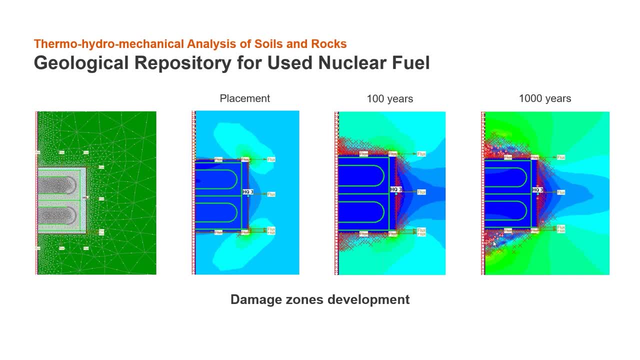 And even in RSU the model didn't converge, So it's implied that the repository were not stable at a thousand years time. It's also implied that the spacings between the room are not enough, and we need to ensure that we can create a spacing between the room to be more than 25 meters. 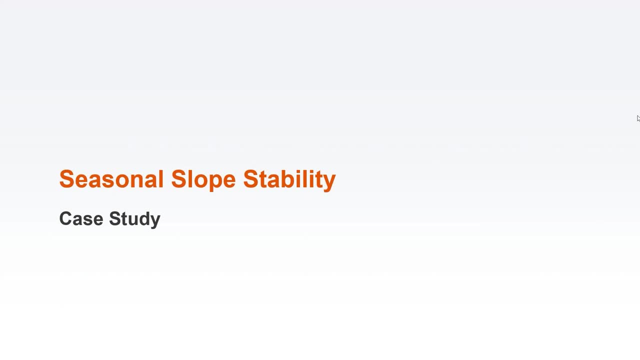 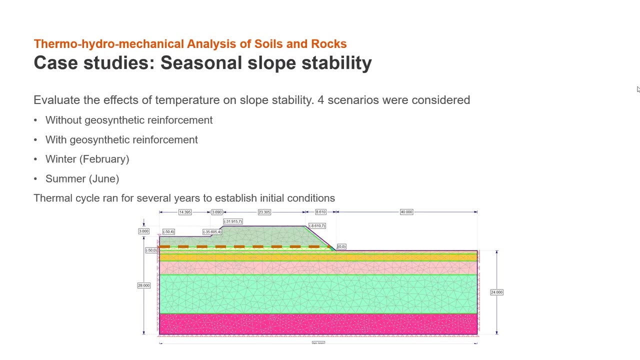 The next application we discussed today is the effect of the seasonal temperature change on the slope stability. This is a very simple models and it's basically a case study when we evaluate the effects of the temperatures and oil temperature changes, and we have four scenarios. 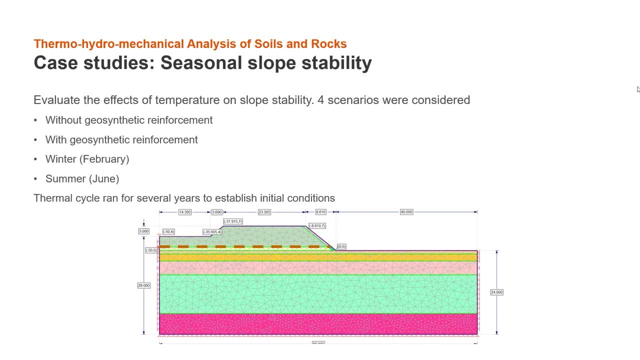 The first one is with the geosynthetic reinforcements. The second one is with geosynthetic reinforcement here. And the first one is we doing the SRF in the winter And another one is in summer. after that winter And for all of the models running the thermal analysis. 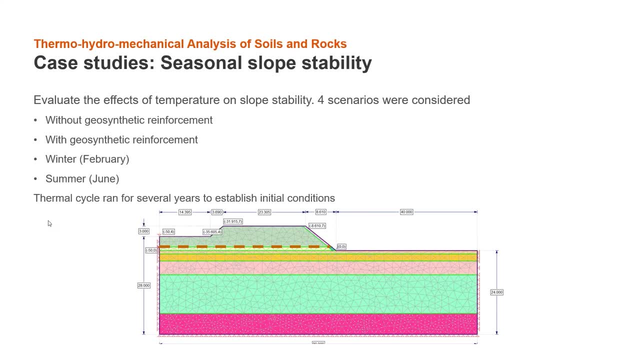 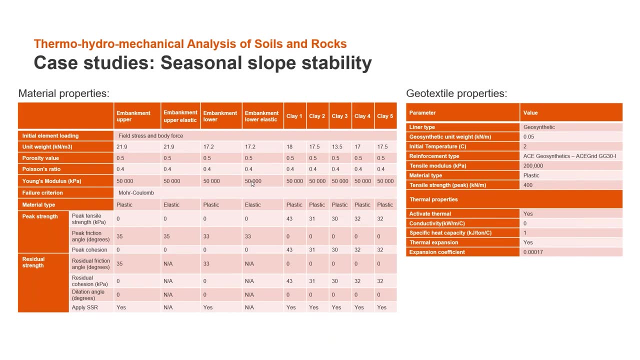 we already run a thermal cycle for several years in order to establish the initial condition. And here is the materials using in the simulation. and it's quite simple. there's nothing fancy, just a regular MOC column with no softening behaviors, zero test type, hyper-tensile strain. 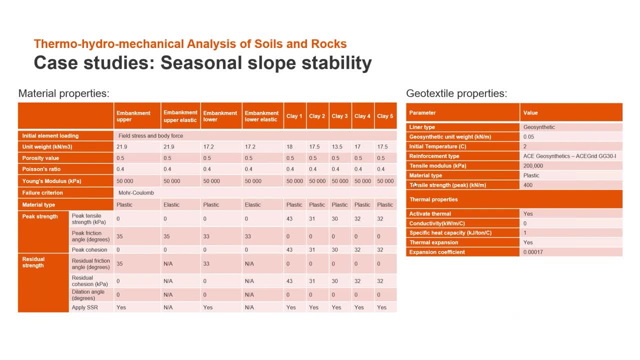 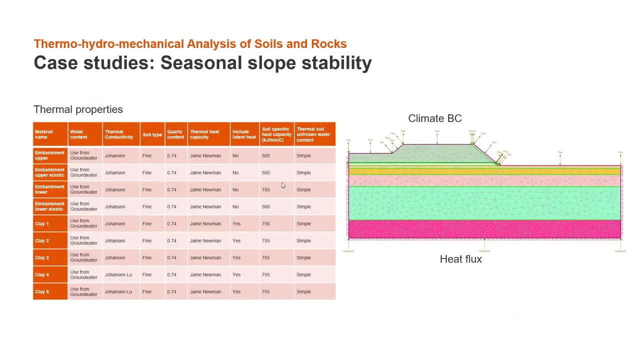 of 400 kilonewton per meters And the expansion coefficient of 1.7 E minus four The thermal properties, which isn't at the typical value for the clay soil. And you can see, here we apply the climate-free condition. 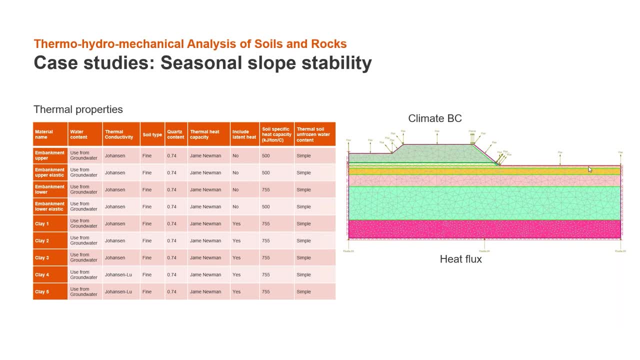 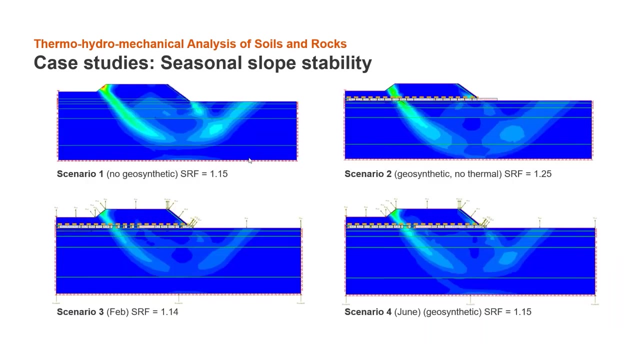 on the top of the models to account for the seasonal thermal changes. The constant heat flux to apply at the bottom of the model to account for the heat transition from the earth or transfer from the earth core. Here are the SRF value from the analysis: 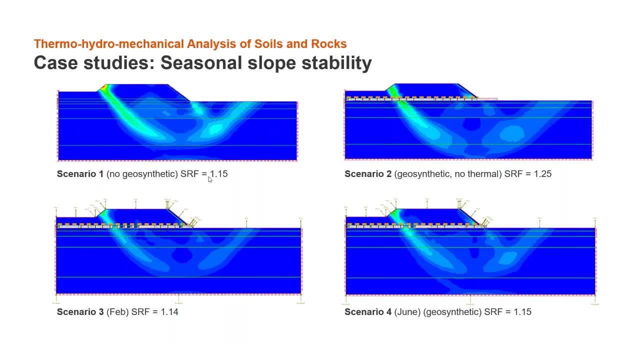 Without the reinforcement, the SRF equal to 1.15.. And the second one: when you install the reinforcement, it increase to 1.25, as expected. However, in the winter the SRF is 1.14,. 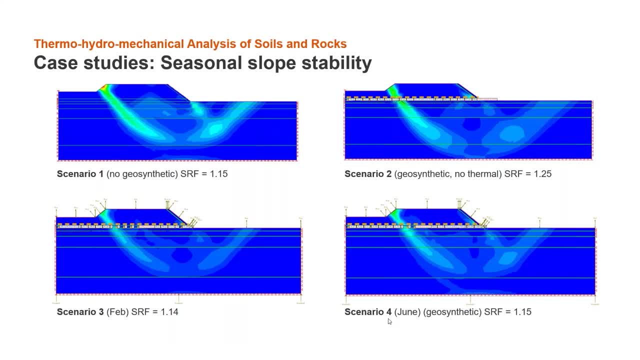 and the summer after that winter it go to 1.15.. It will quite similar, But the difference is that the SRF increase 1.25, and the summer after that winter it increase 1.25.. It will quite surprised for us when we first see the value. 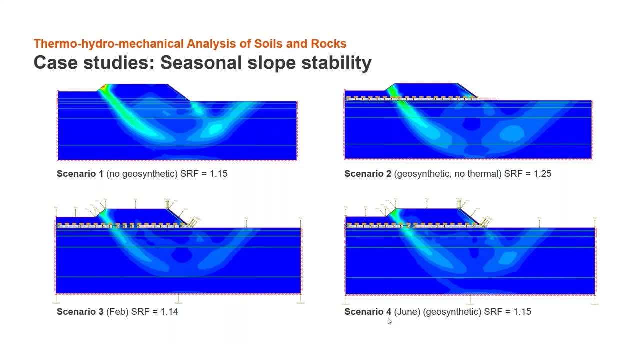 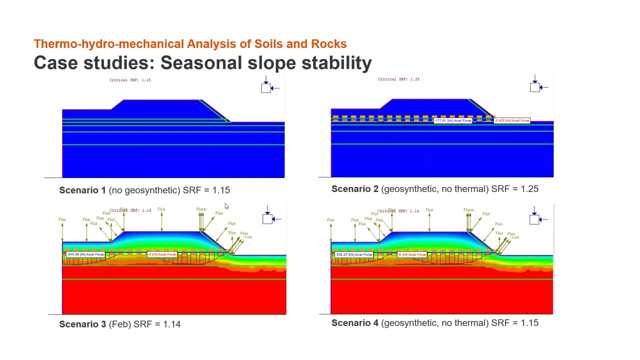 We must think, okay, there's something wrong with the model, There's something wrong with the input parameters. However, we look at the model closer and it quite interesting here. Here is the axial force. When you look at the axial force of the geotextiles. 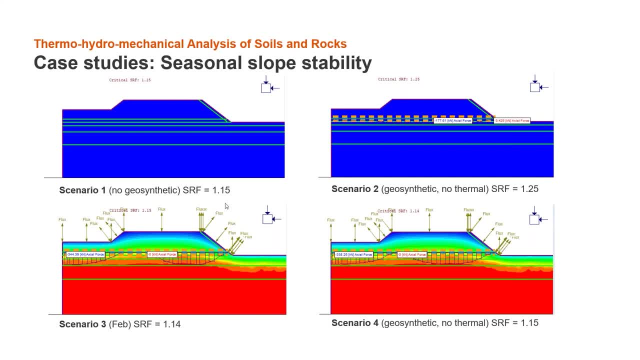 before the safety factor calculation without temperature. In fact, we have the value of the axial force of the geotextiles. Here is the axial force of the geotextiles. Here is the axial force of the geotextiles in tensile force in the geotextile is 177 kilonewtons right. however, here in the winter. 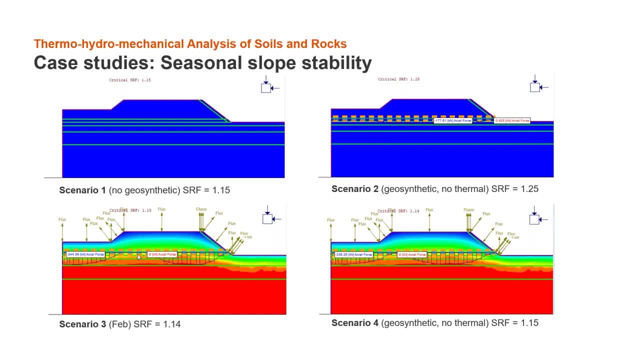 because of the contraction of the geotextile. there are more tensile stress acting on the geotextile. it even exceed the capacity of those textiles at that. you know critical point right here, because they the critical surface right here and it cut through the geotextile right here and 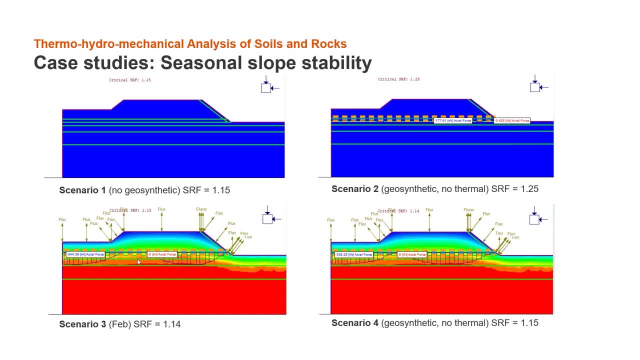 that, on top of the contraction of the textile, is it snapped at that point, and then the slope behaves similarly to one that has no reinforcement and because the geotextile was snapped, it no longer contribute to the stability of the slope in the summer as well, and you can see the 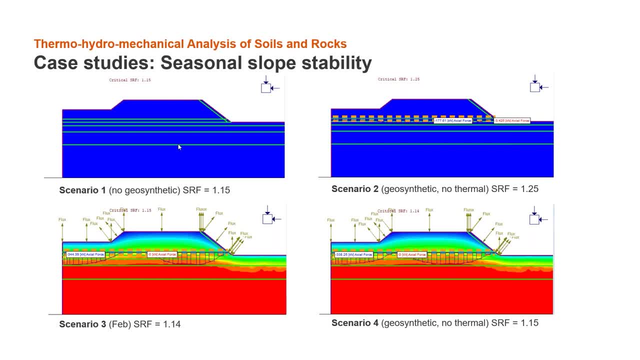 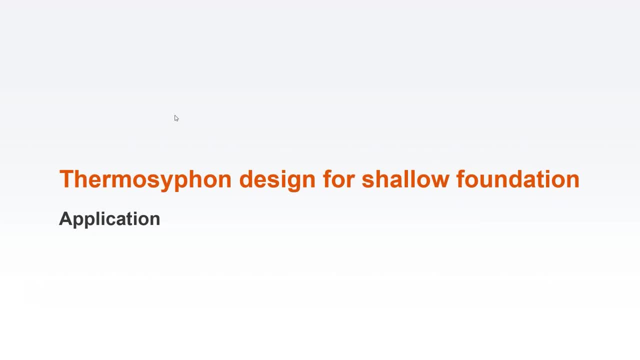 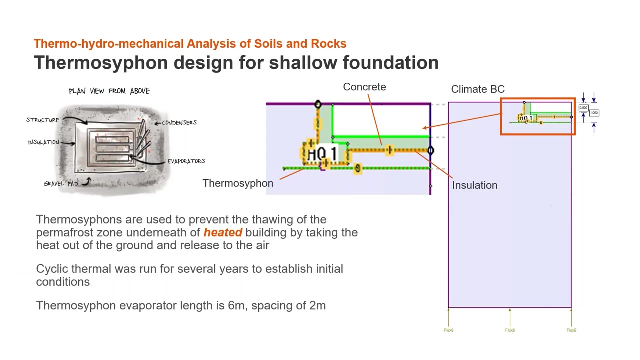 see that the SI value here is just exactly the same, with the SI value here written in the case that you have no geosynthetic equine strategy. The last example I'm presenting today is the design of a thermal siphon for an eye-rich region. So many buildings in the north. 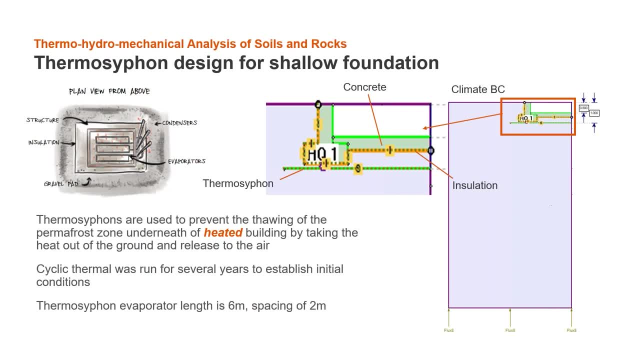 are built on a strong foundation of eye-rich permafrost. because of the climate changes, The air and the ground are granted, as you all know, and following that, permafrost. So the building in the north, right now they are increasingly being built with very expensive, just very expensive. 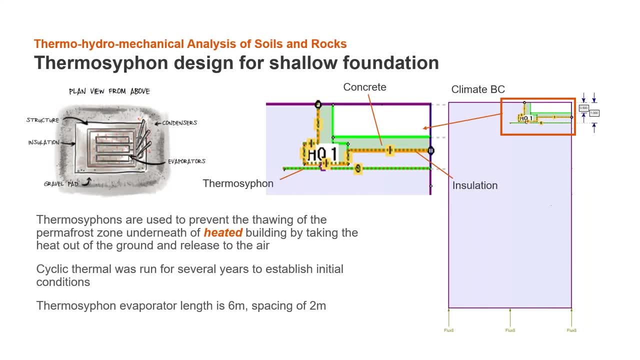 but effective thermal siphon system. In this example we are going to model a flat loop. here's a flat loop: operators, thermal siphons and similar to other models. before installing the thermal siphon: the model will run, with several years to establish the 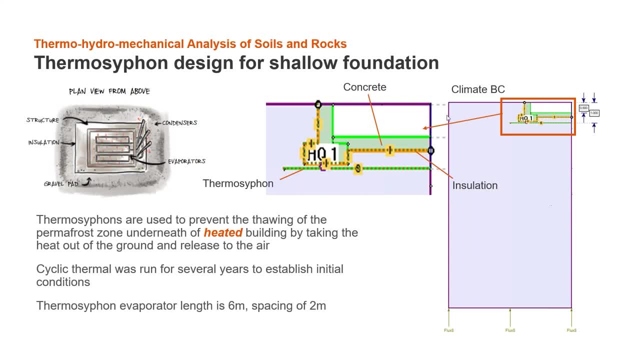 initial temperature distributions using the thermal, the climate condition at the top and the first at the bottom, And after that the thermal siphon were installed one year before the construction of the construction of the foundation, right here, And then the historical report will add underneath of the foundation to monitor the temperature. 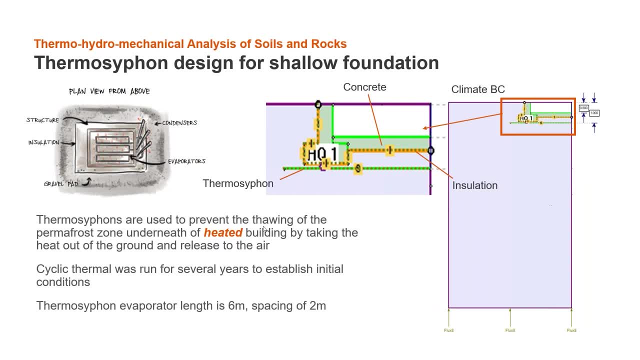 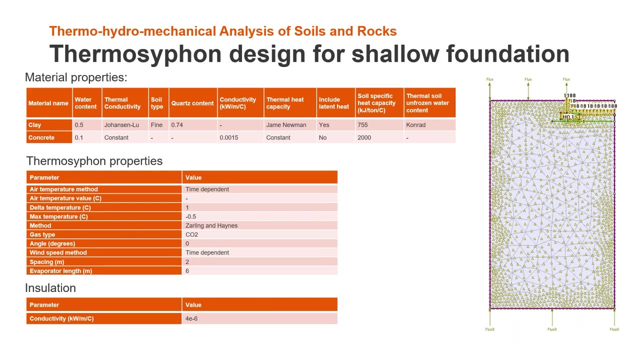 change over time And the purpose of the thermal siphon here is try to keep the soil underneath of the foundations frozen at one time or give it a permafrost. Here are the material strategies in the models of what thermal siphon, which just use zelling and hanging methods with speed and air. 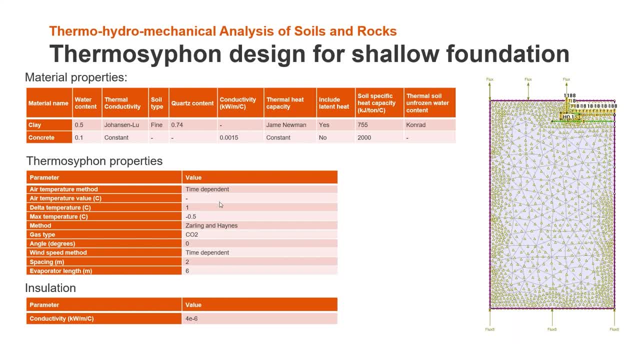 temperatures from the climate variation And we also assign the temperature of aiding to the inside of the concrete foundations to represent the heat and temperatures. And we also have the installation go outside of the foundation here and the conductivity of the insulation is 40 minus six. 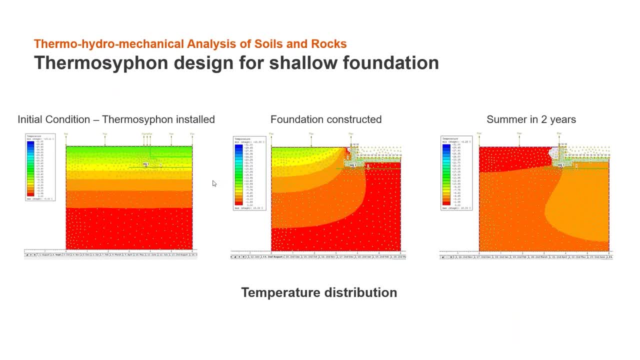 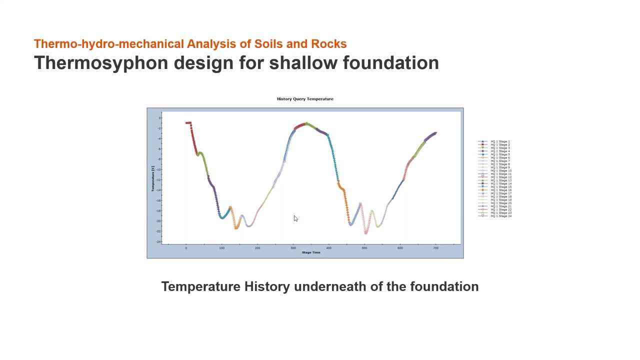 And here is the contour of the temperature distribution here and you can see that from the contour on of the white below the foundations it was frozen for another three cases And we can also look at the temperatures history of that point and you can see that throughout. 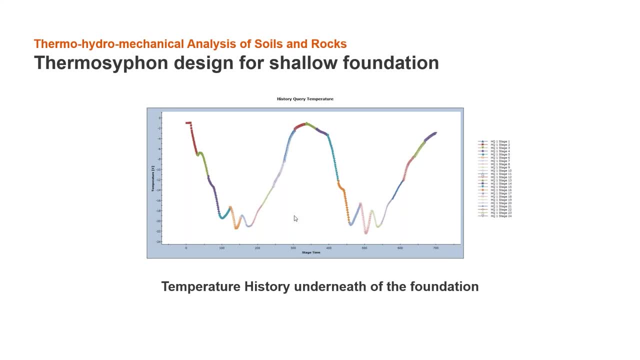 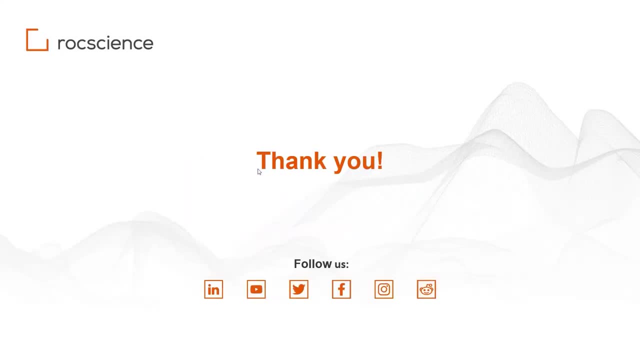 two years, the temperature was always maintained below the frozen point. And that concludes my presentation today, and I will try to answer as many questions as I can, And so let's start with these questions. So the first question, the question I got, is: let me summarize the question: 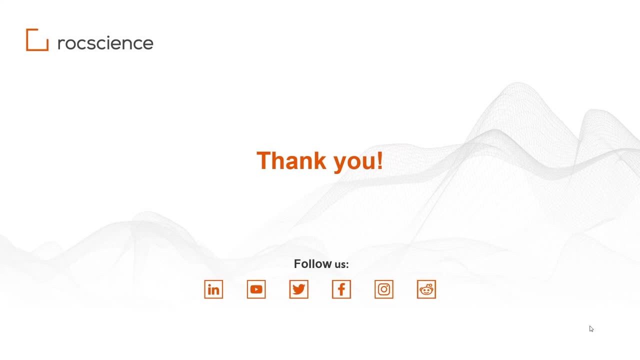 So the question is to see if the change in the strength of the soil is incorporated in IH2.. So that is really a good question, because now we're talking about the thermal induced strength of soil And right now so we have many. actually that's three ways. 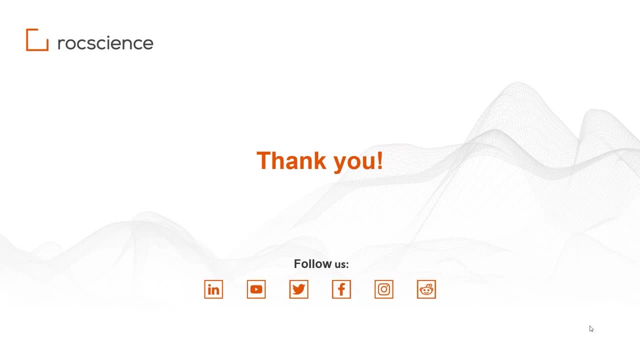 to do that Currently. the first and the most simple way is we're gonna have a function of the property by the temperatures. like, for example: you're gonna have the tabular form of the cohesion changing with the temperatures And as soon as the temperature change. 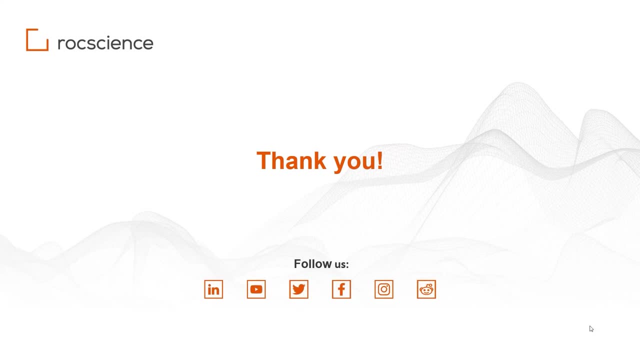 you can just go to the table interpolates from the temperature and get the value that you want. So that is easy And you can do a lot of experiments and data and a lot of work to get that data, But it's simple. The second way to do that is to similar to how we do the calculation for the unsaturated stress, where we don't account for the strength but we account for the stress, similar to the way that we change the strength for the unsaturated soil. 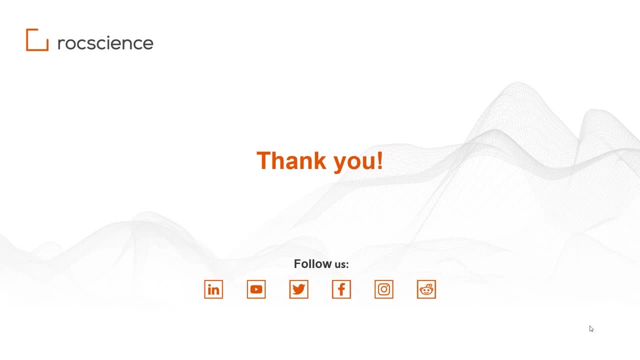 And the first way is we do add a state variable where we consider the temperatures, unfrozen water contained in the soil all together, as in the similar way to that we do with the unsaturated soil models. So, to answer your question in short, we currently actually don't have the capability to 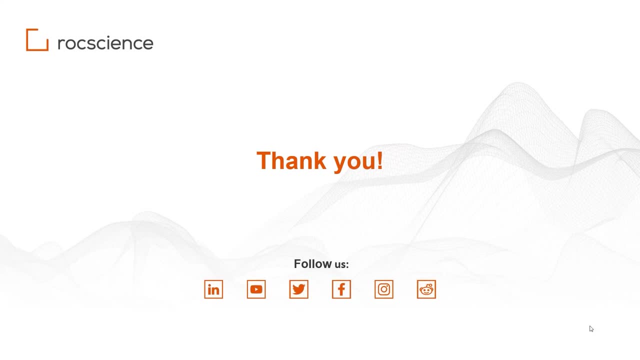 doesn't have the capability to do the state variable approach, But you can certainly input at the tabular form for strain and the temperature change. Okay, so another question I have here is: is there any major difference between the conventional buried foundations used in artificial ground freezing? 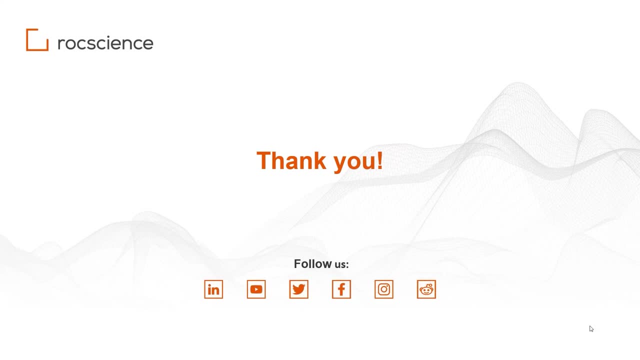 with the end of climate buried foundations used to simulate ground surface in order simulation. So right now you're talking about the two buried condition in IHU. The first one is the convection buried condition And the second one is the climate buried condition. So the climate buried condition actually include the convection buried condition into the system, where it consider the effect of the air temperatures and wind speed to the equation, Whereas the convection system is we consider everything at once and we come up with the heat transfer coefficient. 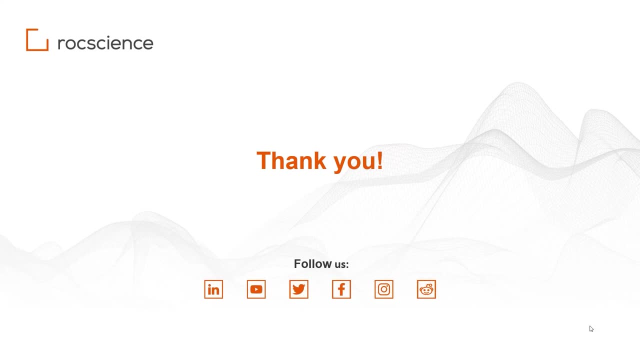 like we call it like effective heat transfer coefficient, to consider every of the effect at once, So both can be used, interchangeable, but the important thing is we need to find the equivalent value to use for both. Does the program account for the air convection?